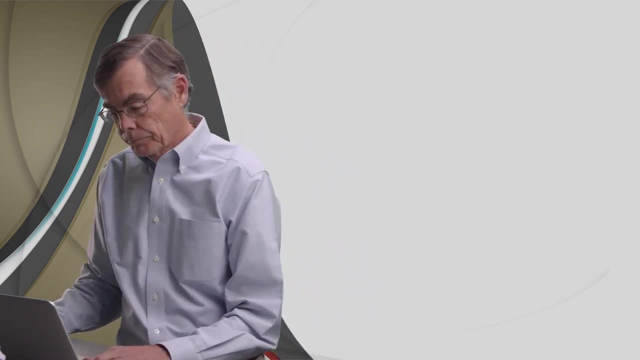 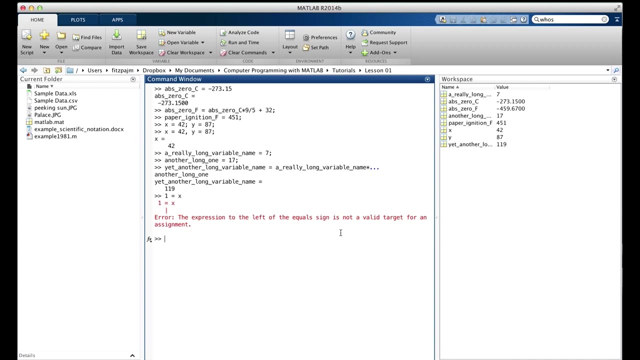 a variable name. Here's another example: One equals x. Of course, MATLAB doesn't like that. As you can see, it says the expression to the left of the equal sign is not a valid target for an assignment. The simple form of this syntax rule. 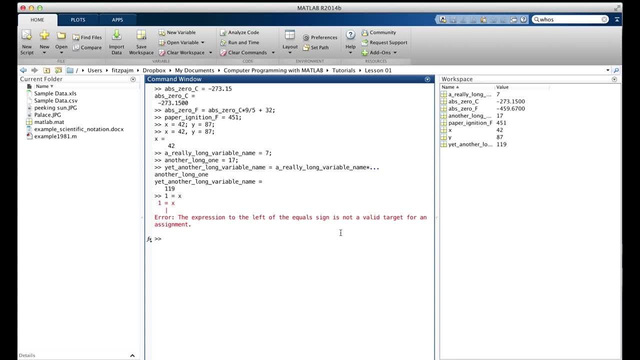 or syntactic rule that we're violating is this: In an assignment statement there must be a variable name on the left of the equal sign. We knew that and we know that one is not a variable name. We'll run into lots more syntax errors as we learn more rules. 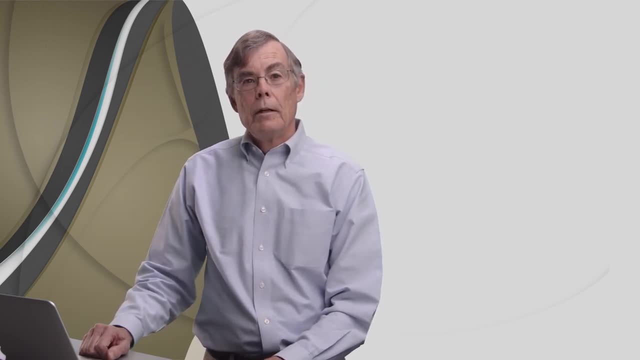 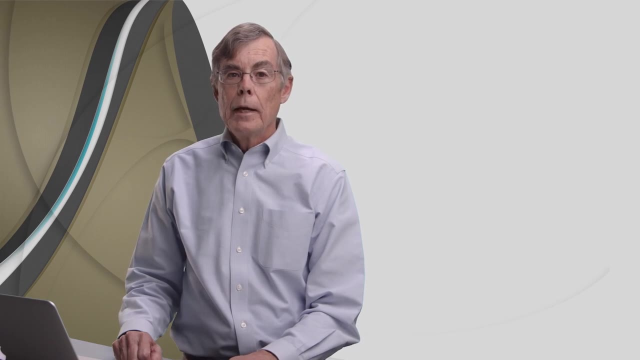 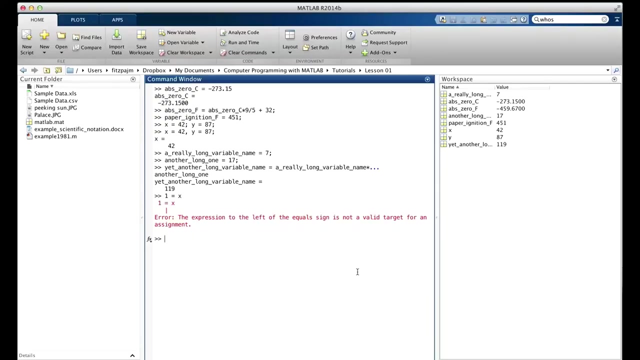 But there's another type of error that is much worse: The semantics error. As we said, the syntax of a command is its form, The semantics of a command is its meaning. An example of semantics is this: Suppose we want to swap the values that are in x and y. 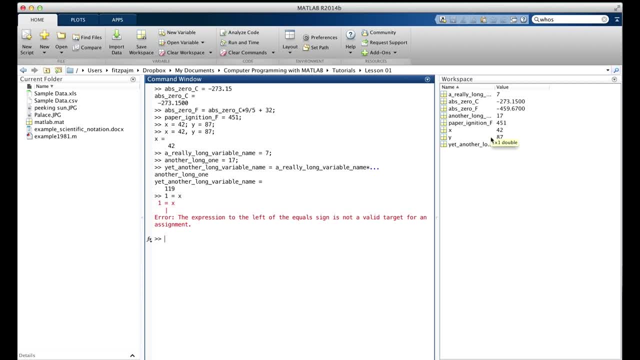 First note that the current value of x is 42 and the current value of y is 87. I've seen many new programmers try to do it like this And, by the way, I'm certain I did it too when I was starting out. 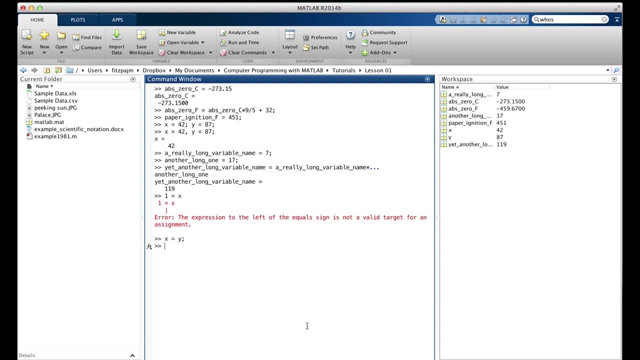 So the type x equals y and y equals x. You see what went wrong here. Let's look up here and see that something did go wrong. They're both equal 87.. Instead of having their values swap, they both now have the value that y had before. 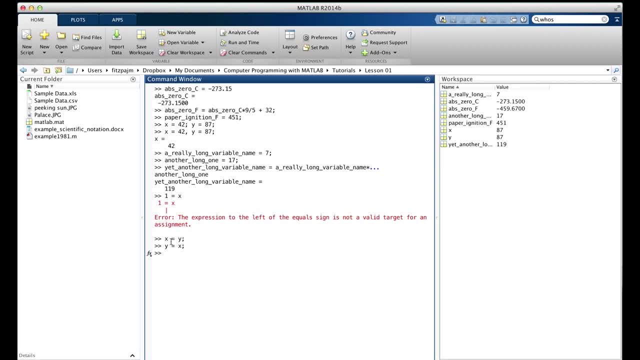 So what happened? Well, the first statement, this one here, copied the 87 that was in y into x, And at this point they both have the value 87. So x's value has just been lost. 42 is gone. 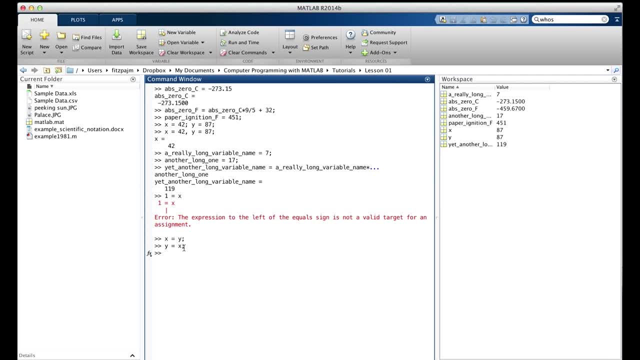 So x's value has just been lost, 42 is gone. Then this next statement just copies whatever's in x, which happens to be 87, now back into y. So y is 87,, it was 87,. that really didn't do anything. 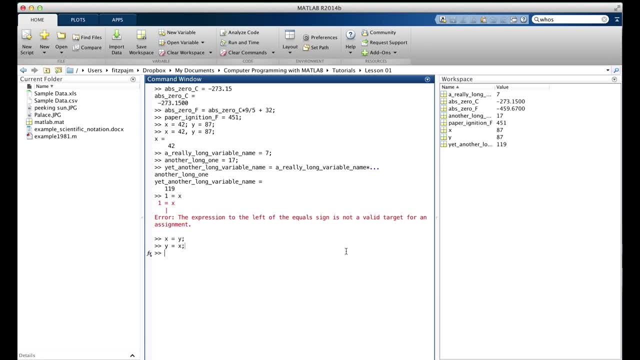 Well, let's do it right. First, let's set things up the way they were to begin with: X was equal to 42, and y was equal to 87. And we can see that we've done that over here in the workspace.